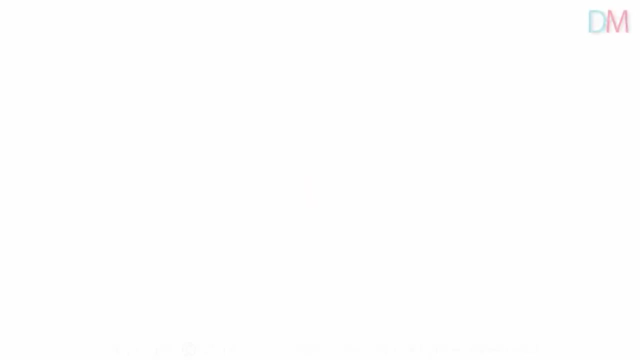 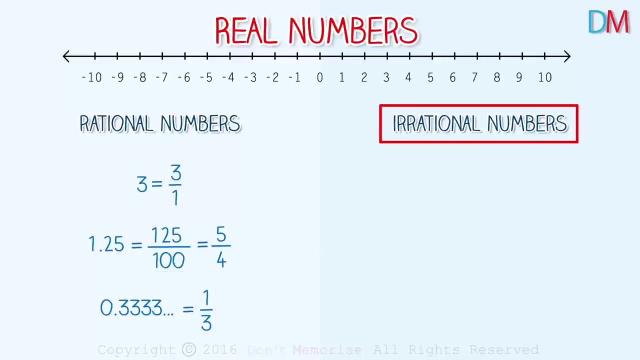 We already know what real numbers are. These are the numbers that can be represented on the number line. We also know that real numbers can be broadly classified as rational and irrational numbers. Rational numbers are those that can be represented as ratio of two integers with no common factor. 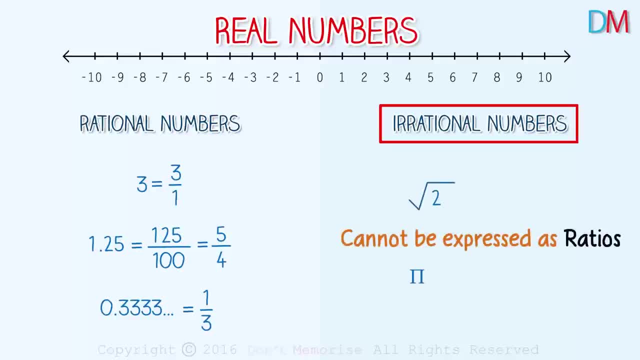 Irrational numbers, on the other hand, cannot be expressed as ratio of two integers, and when expressed in decimal notation, they are non-terminating, non-recurring decimals. Are there any other kinds of numbers, Numbers that we haven't looked at yet? 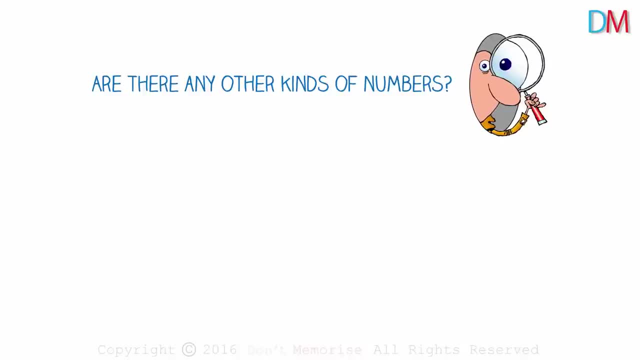 Before you answer that question, let me ask you another one. Can you think of a number which, when squared, results in a negative number? Yes, a number which, when multiplied with itself, gives a negative number. Try it. You'd have probably tried a few options. 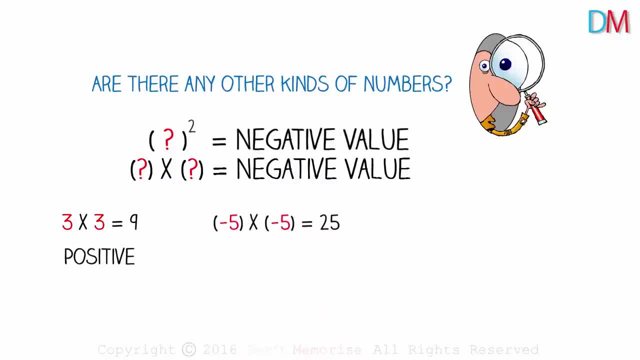 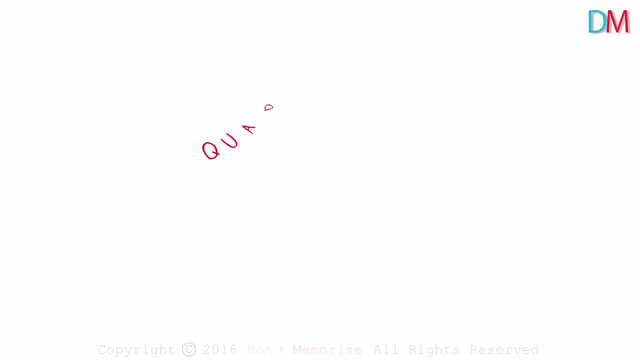 Three times three is nine: positive Negative. five times negative. five is twenty five again positive: Negative root three times negative root three is three positive, again No luck, We'll come back to this, don't worry. So we've studied quadratic equations in middle school. 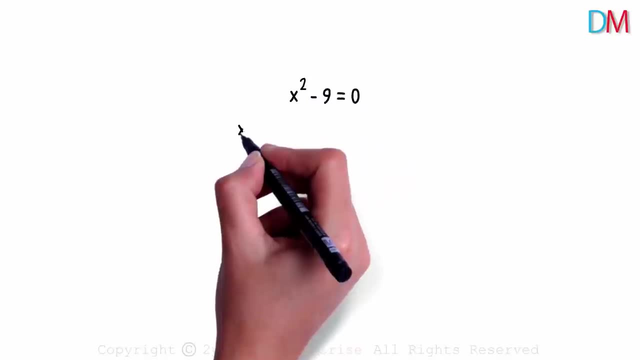 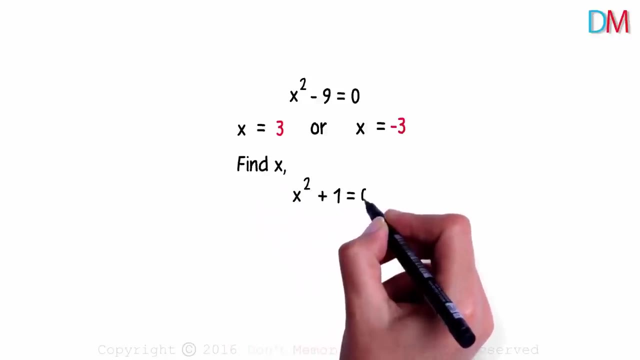 We know that if X squared minus nine is equal to zero, X is either equal to three or negative three. Now try to find a solution to X squared plus one, equal to zero. Not sure, Or do you think there's no solution to this one? 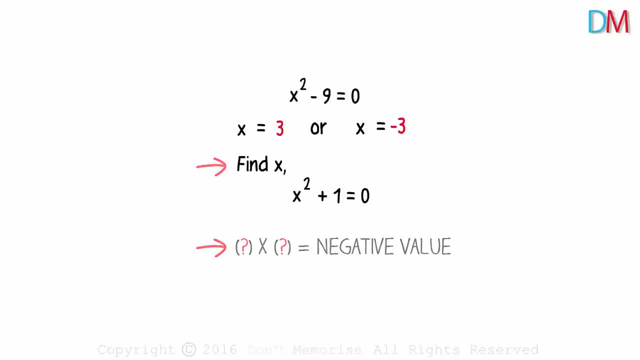 Don't worry if you couldn't get the answer to these two questions. Let's understand the situation now. Whenever we considered the square of a number, say X, the result was always positive, whether the number X was a positive real number or a negative one. 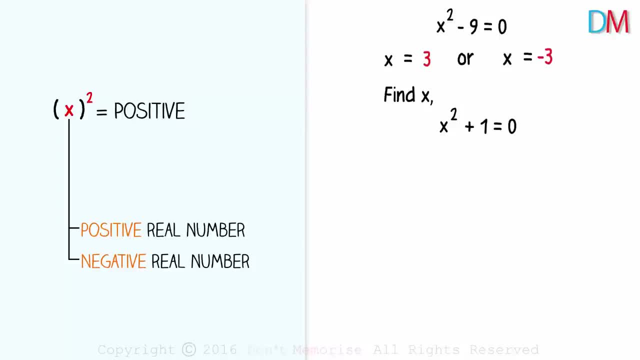 We always got a positive result And we had learnt that a negative number did not have a square root. So if we had a number like negative nine, we said that its square root did not exist. Do you remember that while finding the solution of a quadratic equation using the formula, 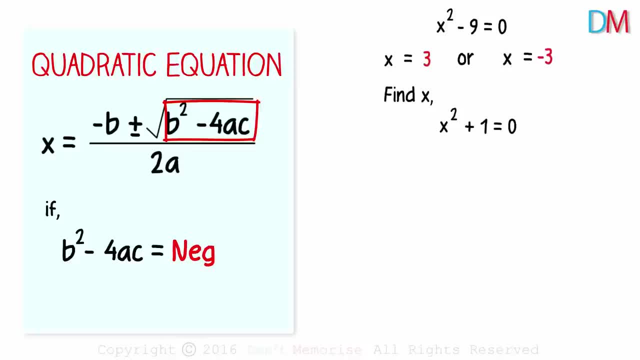 if the discriminant B squared minus four AC was negative, we said that there are no real roots of the quadratic equation Based on what we had studied earlier. X squared plus one equal to zero is negative. X squared plus one equal to zero will not have any real roots as the value of discriminant. 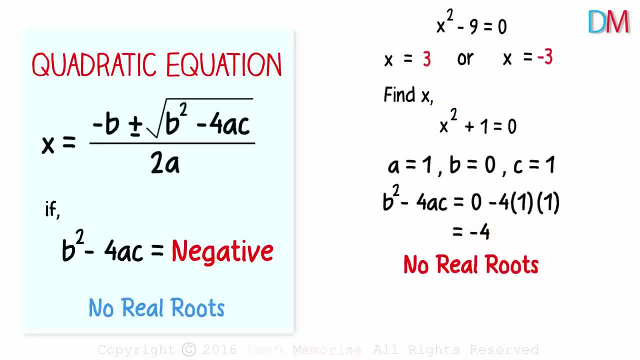 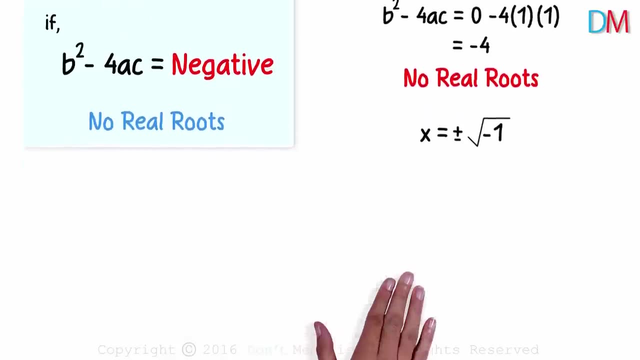 is negative four. Why did we do this? What was the problem here? It's easy. As the square root of negative one did not exist for us, we said that there was no solution for the equation: X squared plus one equals zero. However, in the 16th century, it was a mathematician named Cardin who first started thinking about 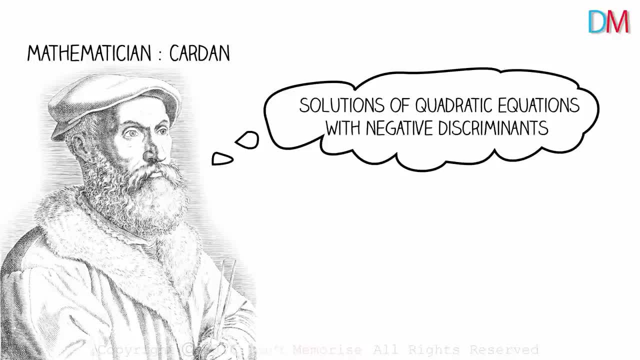 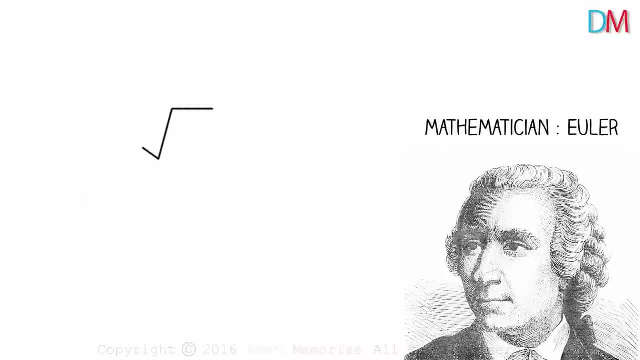 solutions of quadratic equations. He used quadratic equations with negative discriminants. Soon others started too. but it was Euler, in the 18th century, who gave the square root of negative one a symbol, i, and called it the unit imaginary number. These were termed so as they were thought to be impossible and just something we imagined. 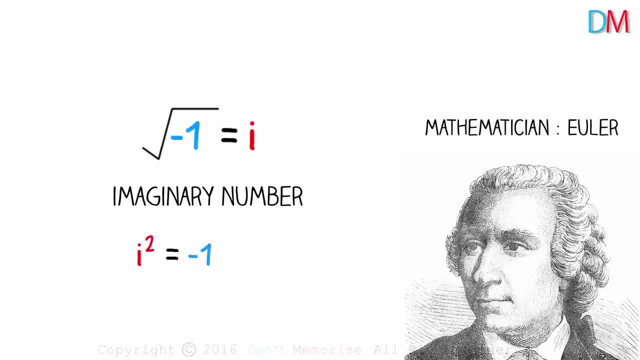 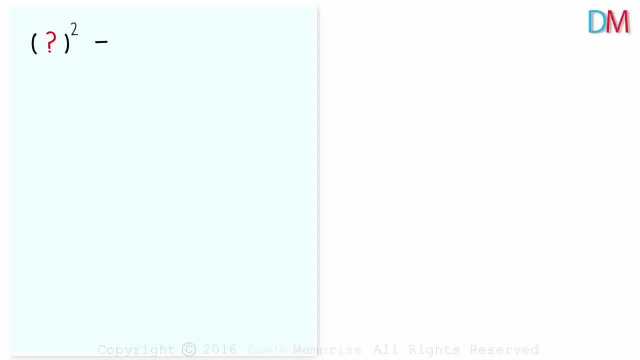 So i was assumed to be a number whose square is negative one. Now you'll be able to answer the two questions. Can you think of a formula, Can you think of a number which, when squared, results in a negative number? Yes, It's i. 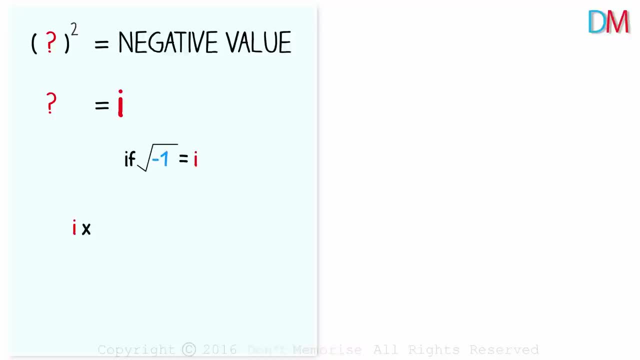 If square root of negative one is i, what is i times i or i squared, It is root negative. one times root negative one, That gives us negative one. There you go: We got a negative number by squaring a number. And the next question was: can you find a solution to X squared plus one equal to zero? 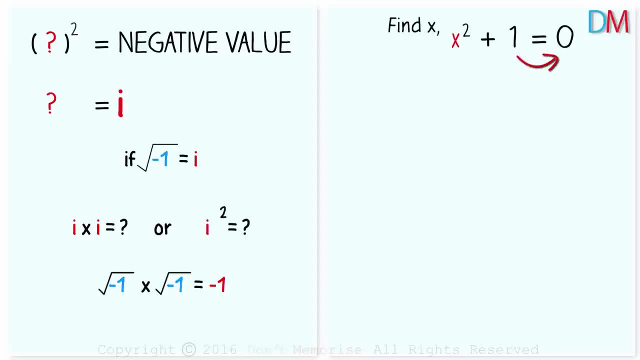 The answer is yes. Transposing one to the right hand side, we get X squared as negative one. Taking the square root on both sides, we get the value of X as root of negative one or minus root of negative one. That is plus minus i. 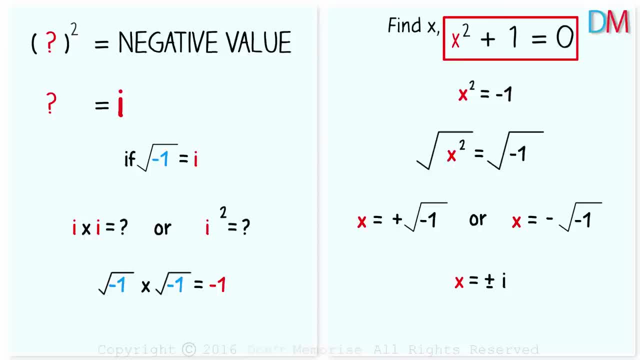 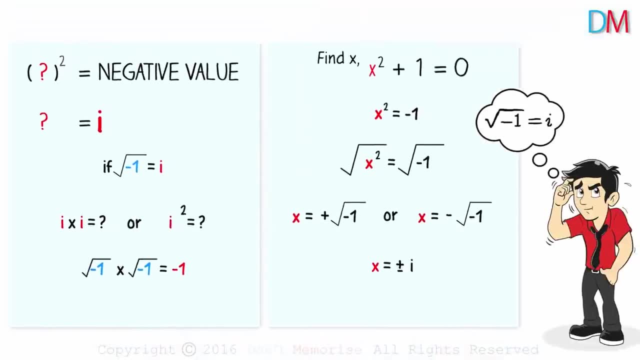 So what we learnt in school wasn't incorrect. This equation has no real roots. Yes, it has imaginary roots. That's the concept of imaginary numbers for you, Thank you. But wait, we understood the concept of square root of negative one.